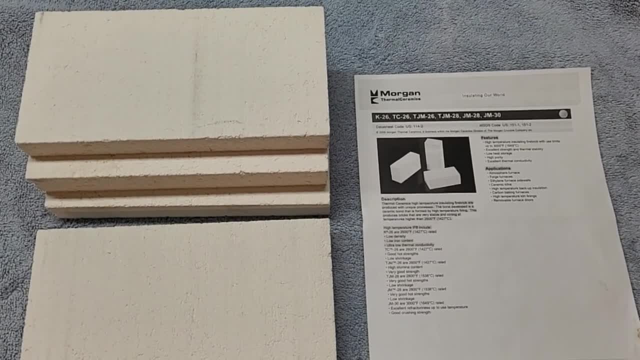 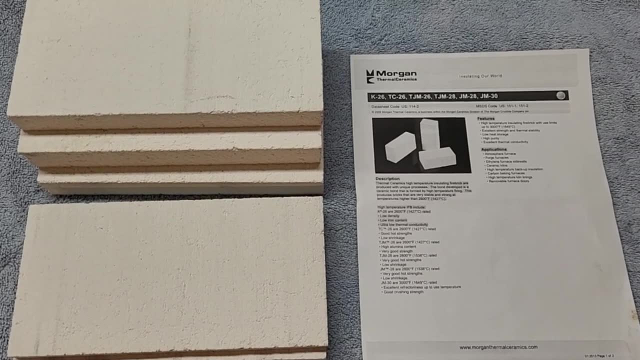 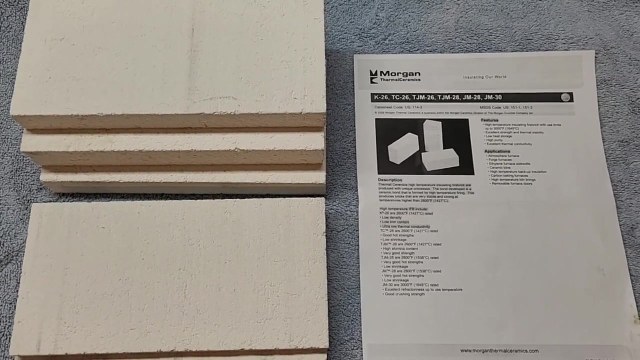 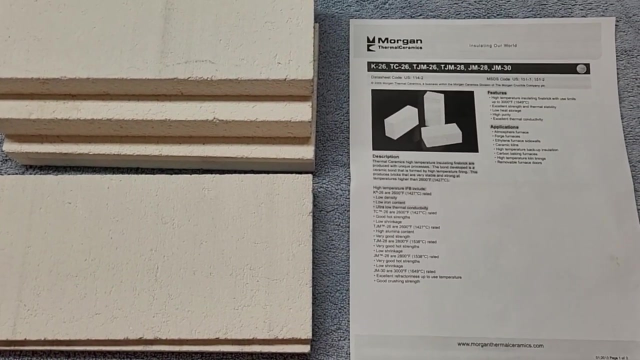 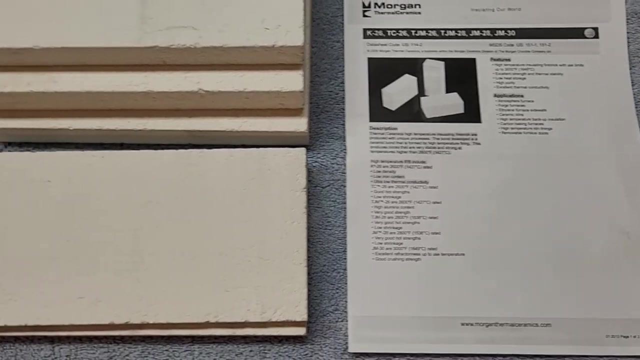 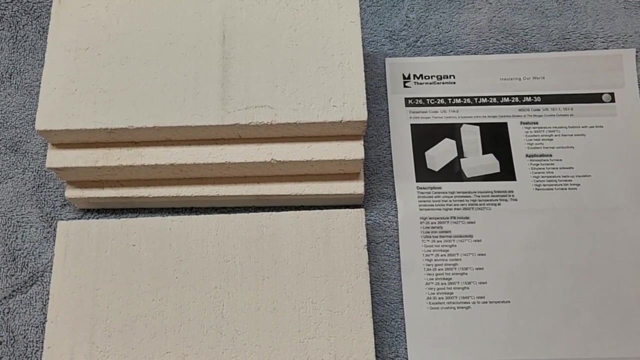 Hi, this is a quick review of some Morgan Thermal Ceramic Insulating Fire Bricks that I got from I Ya Knows Best on Etsy. I'll post a link to their store so you can look at the specifications for the bricks And I'll also post a copy of the spec sheet that you see here. that gives all the details about these bricks. The reason I wanted to take a look at these bricks is that they are advertised as insulating bricks as opposed to fireplace bricks. 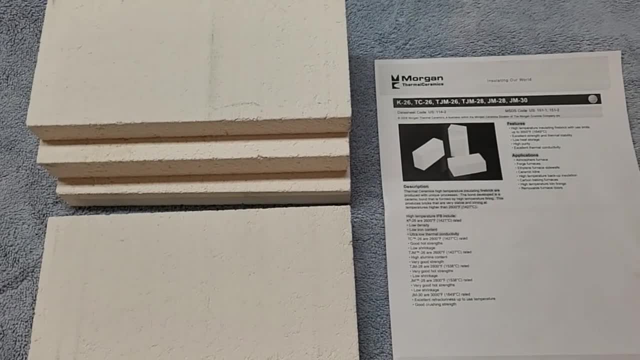 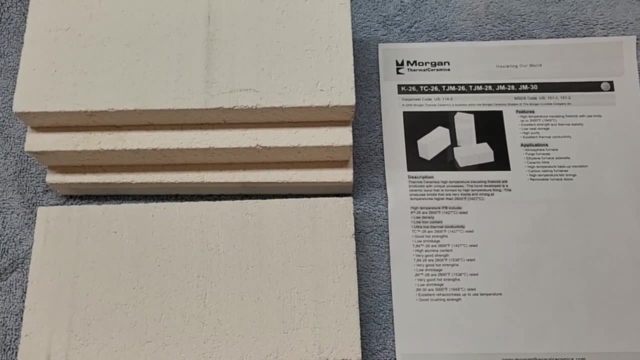 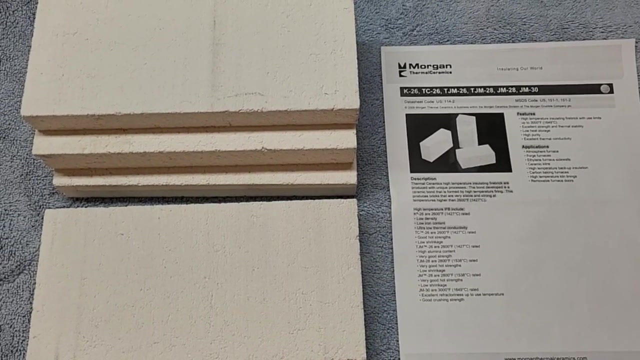 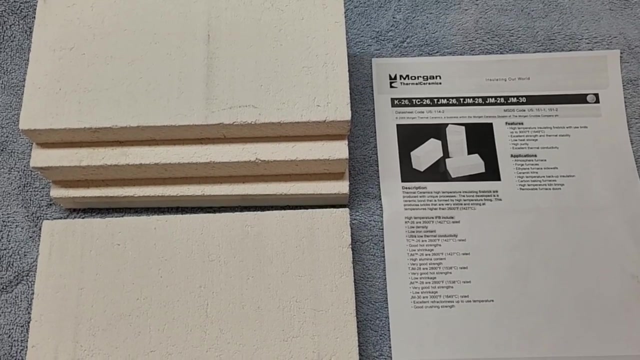 So I've been using some Rutland fire bricks and they've worked pretty well. I'm not complaining about them, but I wanted to try these because the people over at I Ya Knows Best said that these should actually perform better, simply because they are insulating as opposed to absorbing the heat from your forge. 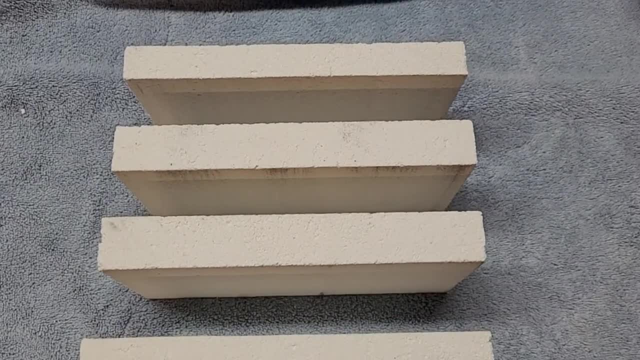 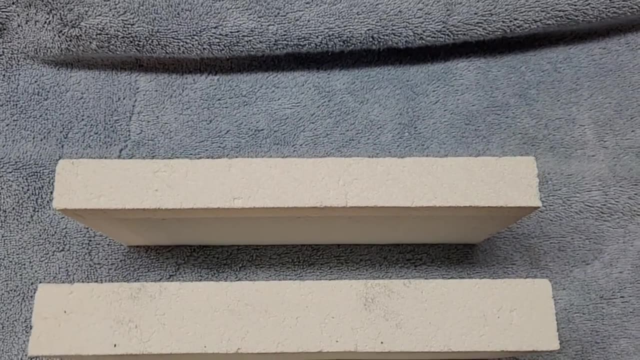 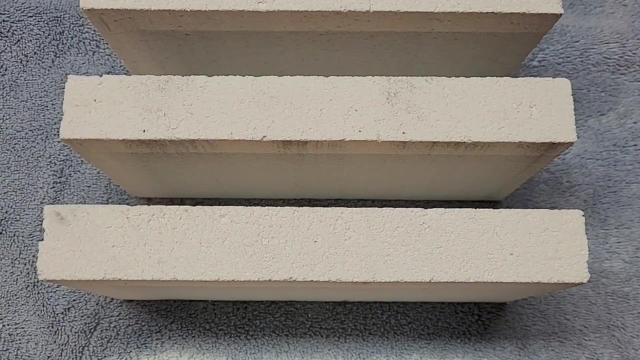 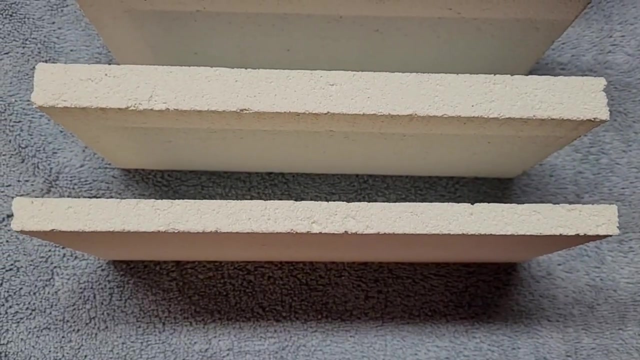 I have several different sizes here. I have a standard 4.5 by 9 inch. Here in the back I have a couple of 4.5 by 9 inch, by inch and a quarter, And then also I have a 3 quarter inch and a half inch thick brick that I'm going to give a try. 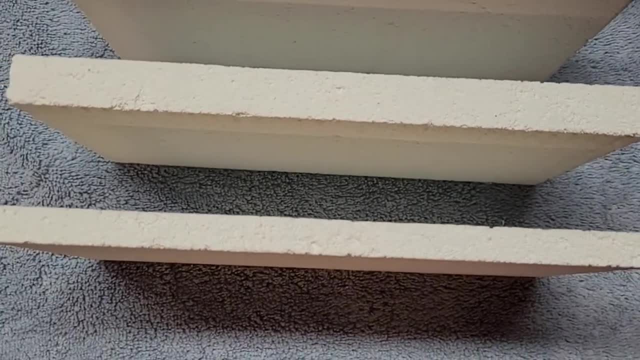 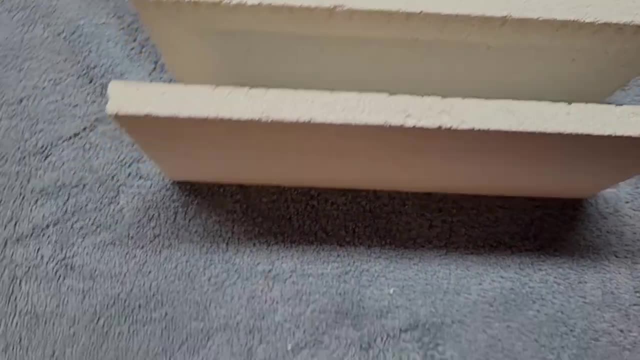 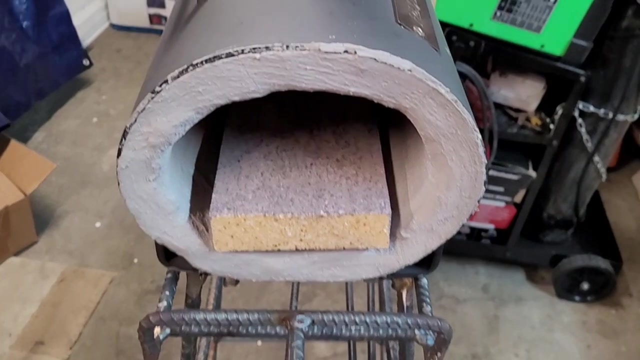 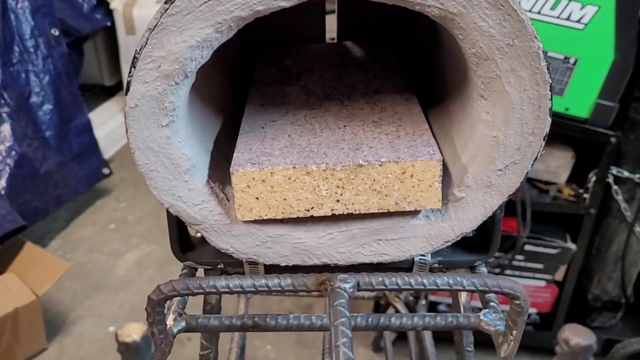 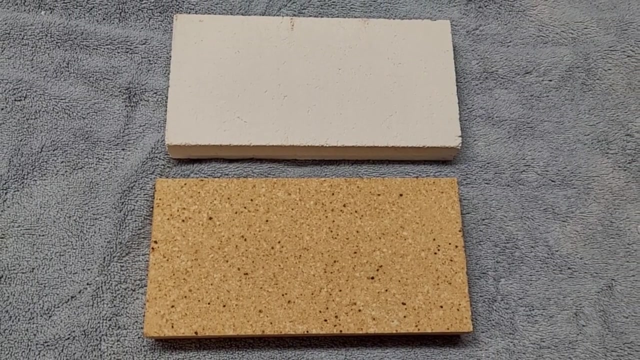 What I like about the last two is that, you know, given that they're a little bit thinner, it gives me a little bit more space in my forge And I'm using- I'm using- a Hell's Forge single burner forge that you can see here and it works great for my stuff here in my little home shop. but you know, it's good at some point to have a little more extra space in there to work on a little bit larger items. 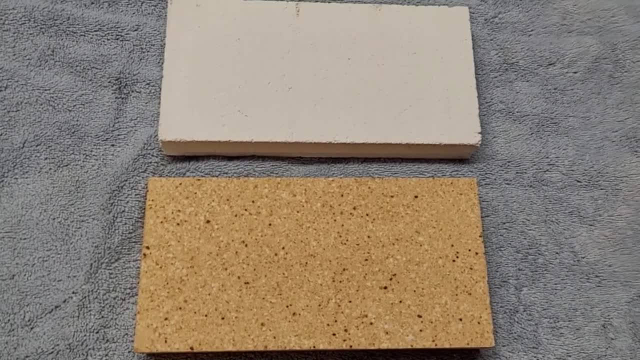 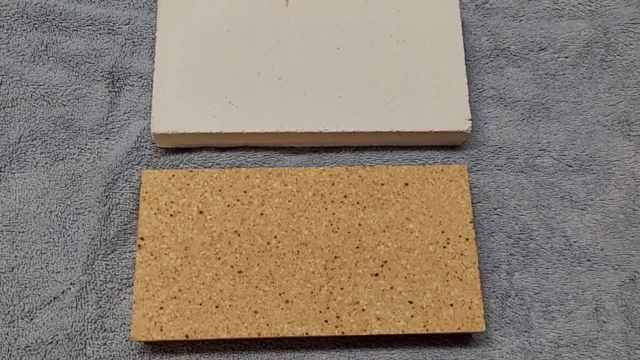 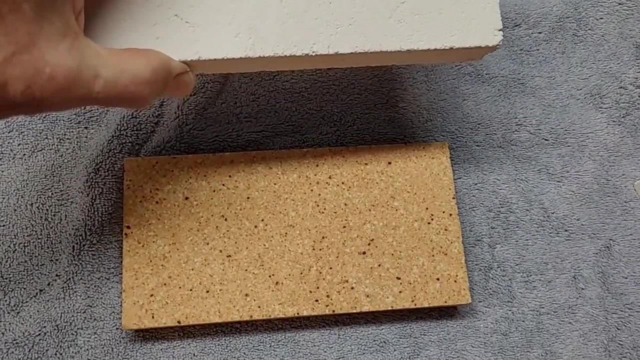 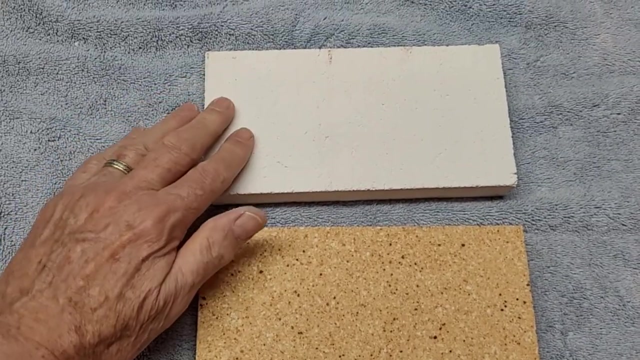 So this is a side by side comparison of one of the Rutland fireplace fire bricks. The first thing you will notice about these bricks is that, compared to the Rutland brick, the Morgan thermal ceramic brick seems a lot less dense and therefore a lot lighter. 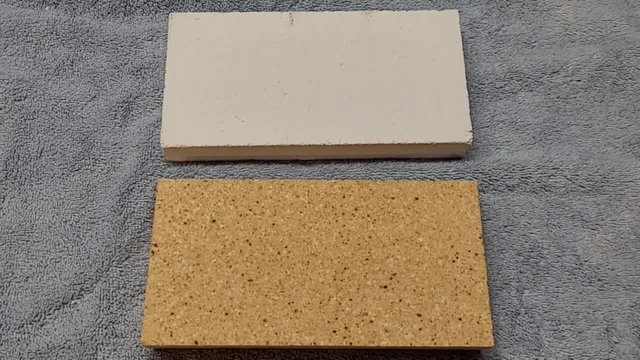 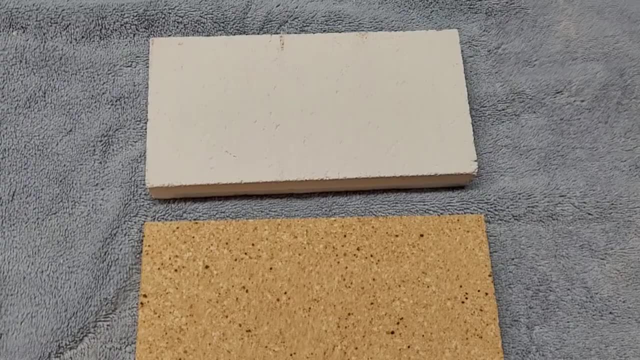 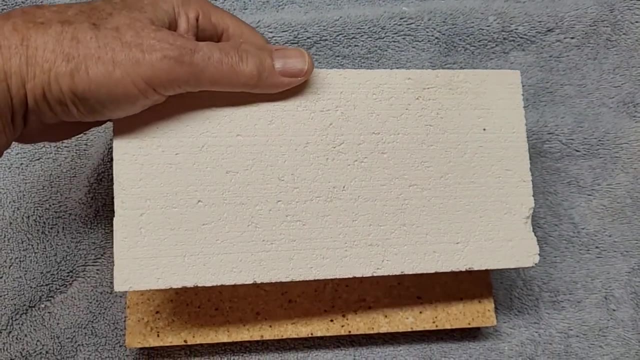 But again, it is an insulating brick as opposed to a fire brick. So you know, if you kind of think of space shuttle insulating technology, Those insulating tile tiles were very light and you know, this brick from thermal ceramics is very light compared to the Rutland. 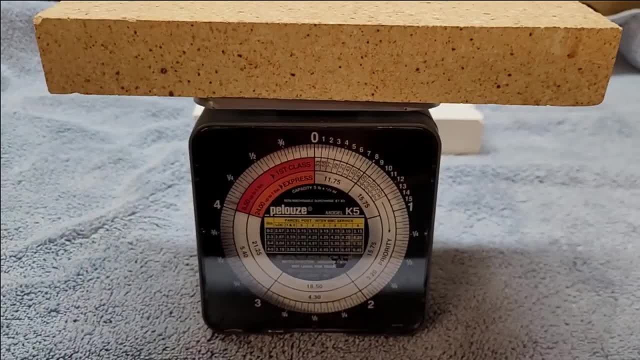 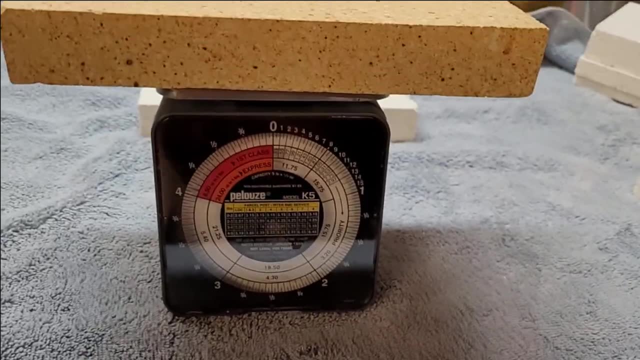 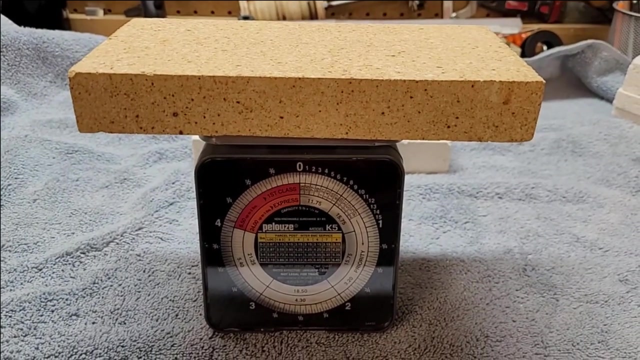 In fact, let's put them on the scale and see the difference. So this is the Rutland brick on my scale and you can't really see the needle too well, but it's right over here. So it's just over four pounds for the four and a half by nine. 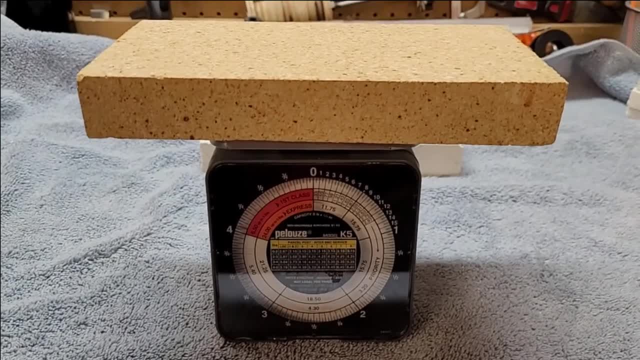 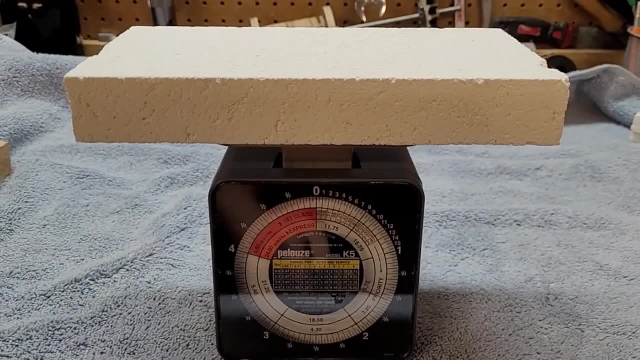 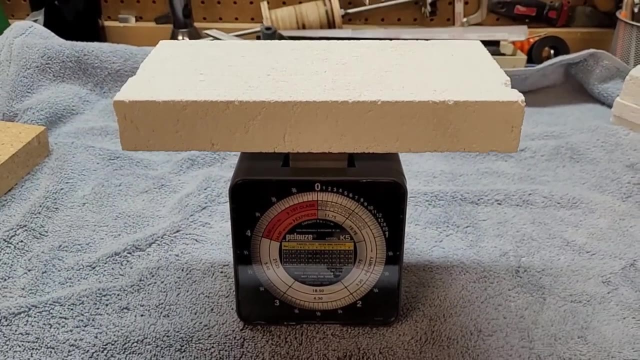 By one and a quarter inch brick. So this is the Morgan thermal ceramic insulating fire brick And you can see right out here we're in at about a pound and a half, So it's significantly lighter than the Rutland fireplace fire brick. 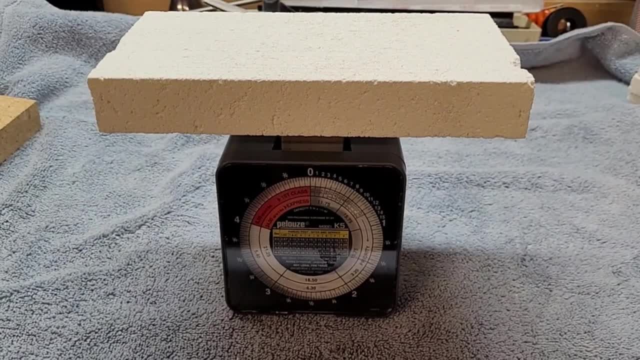 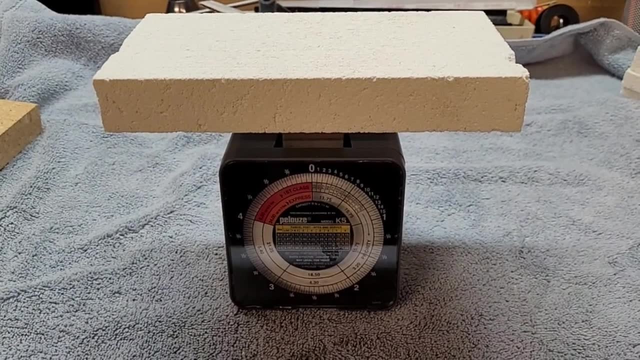 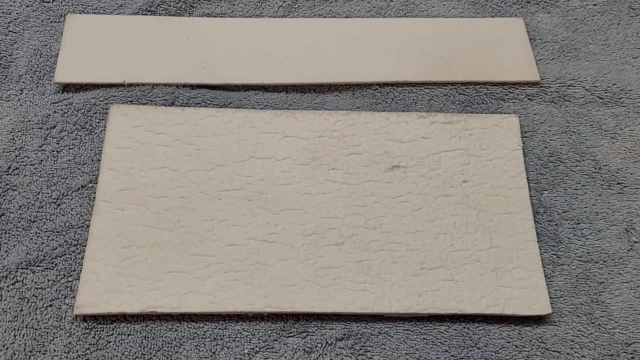 And you know, one advantage of that is, when you're moving your forge around, It's just a little bit lighter weight to have to deal with. I've also got a couple of pieces of kale wool- I'm not sure I'm saying that right. k-a-o-w-o-o-l from I, you know, is best and 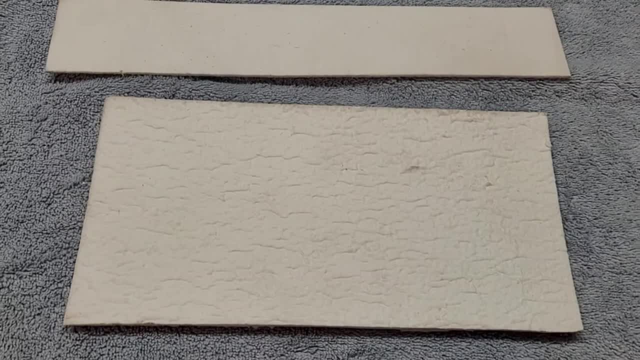 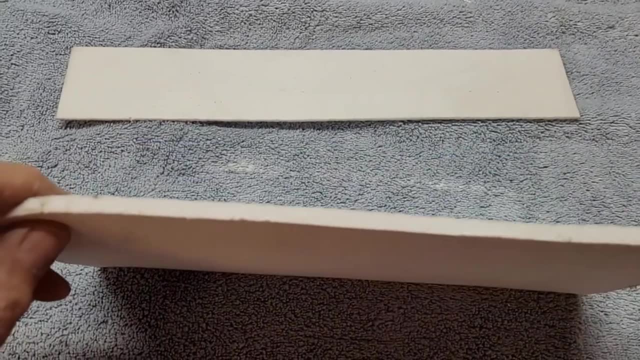 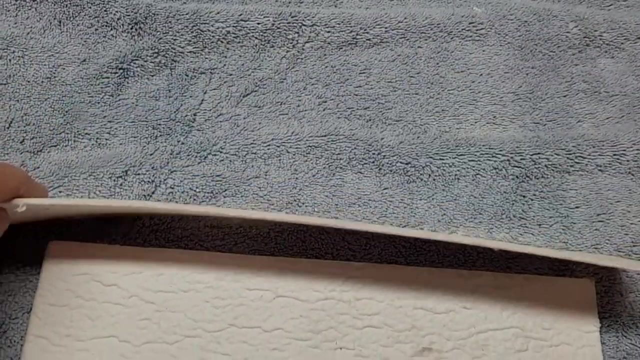 this is thermal wool paper. they call it insulating paper, and it's different thicknesses, as you can see. you can cut it, shape it to any size you want. what I'm going to do with it is use it to seal the small gap between the bricks in. 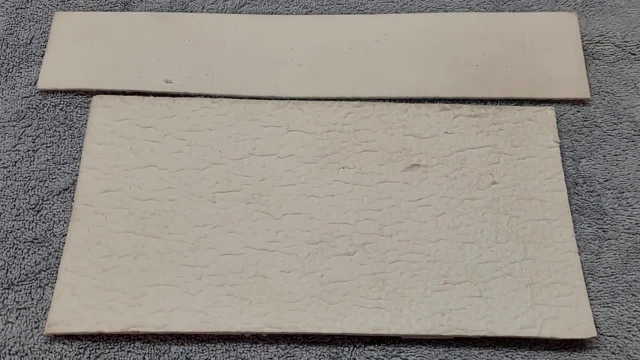 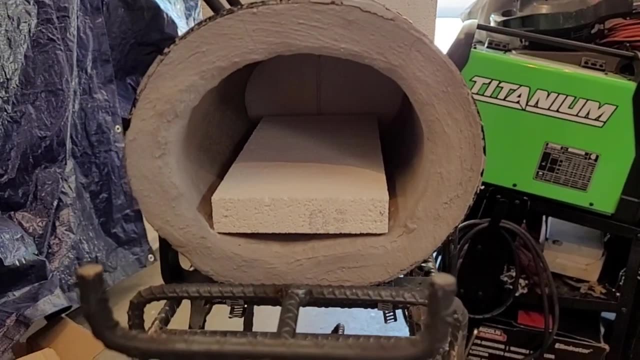 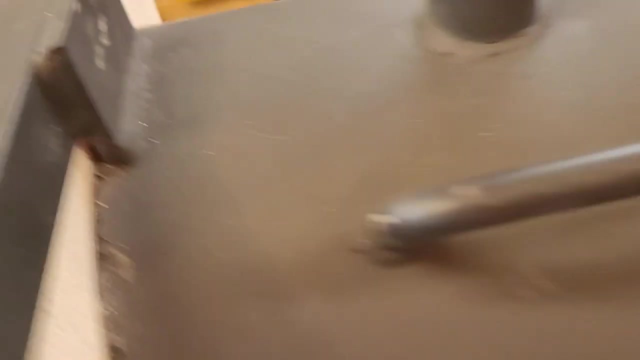 the back of my forge, just as a little bit of extra insulation back there and to seal off the airflow, I've got the one inch thick insulating fire brick inside my forge and then to seal it off in the back, I've got the two inch and a quarters and, as you can see right here, 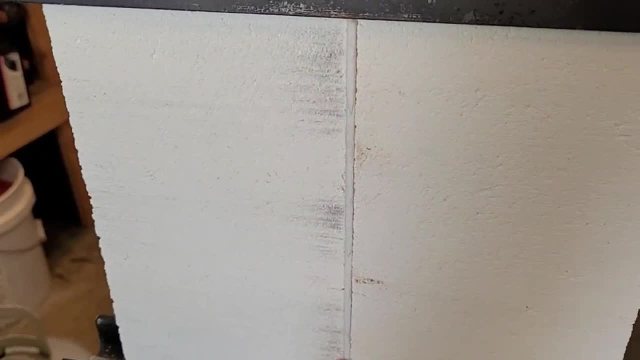 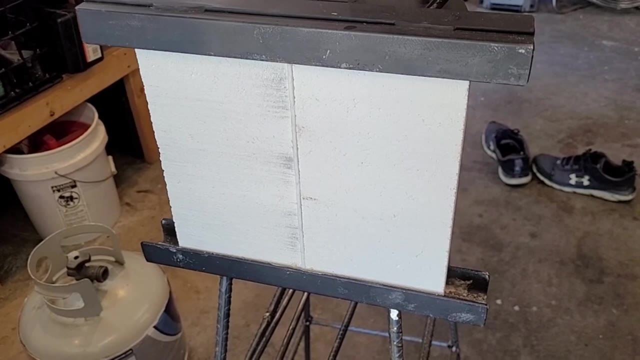 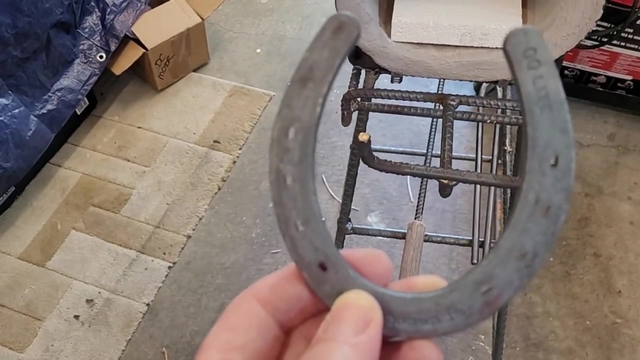 I've got the insulating kale wool paper in between them, so now I've got a really nice tight seal to prevent any air leakage out of the forge. so as a test I'm going to use a zero, zero light horseshoe that I get from National. 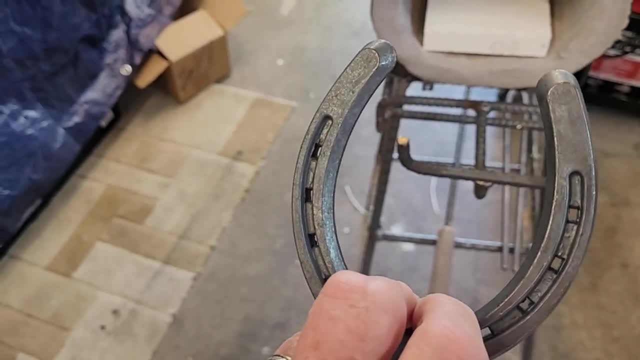 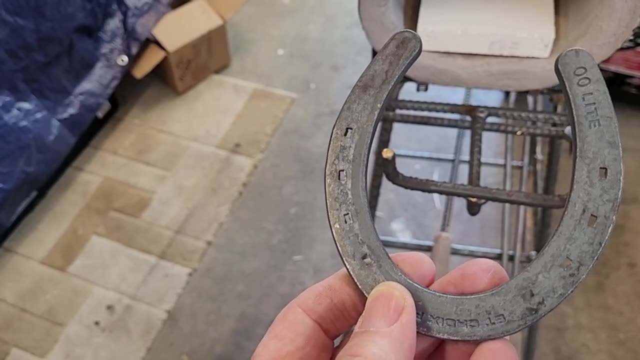 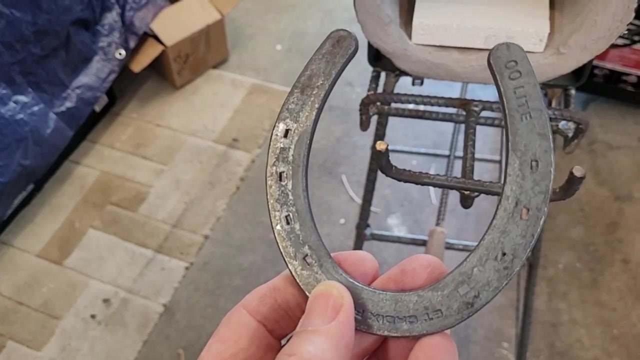 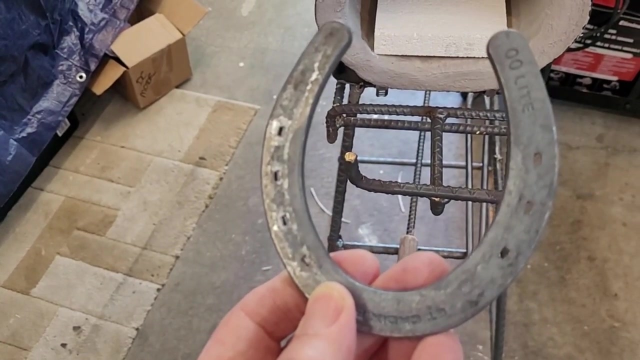 Rodeo Supply. I use these a lot. I use these a lot in my yard art work and it typically takes about, I would say, between four and five minutes to heat one of these to a temperature where I can bend it in my vise or on an anvil. so I know this is not a terribly scientific test, but 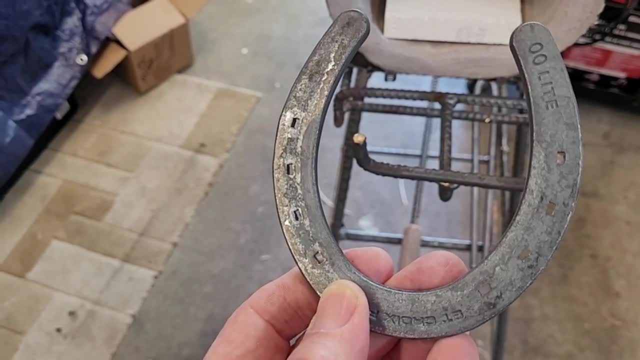 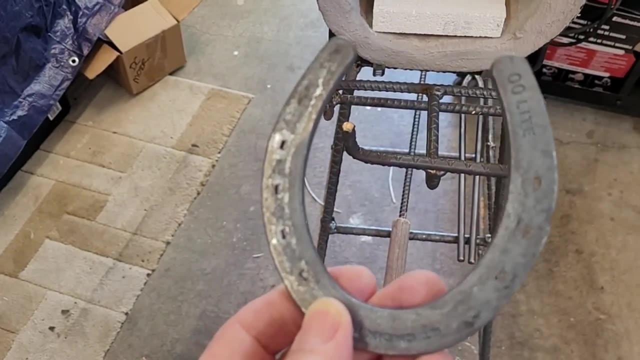 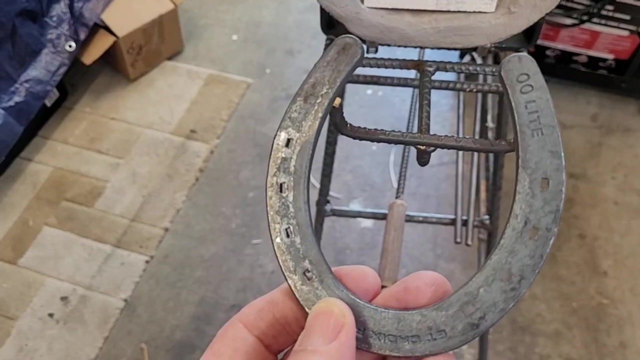 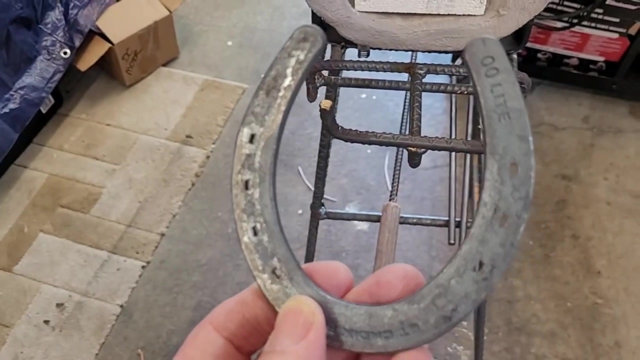 anyway, we'll give it a see and see if there's any significant difference between these insulating bricks and the regular fire bricks. but what I would expect is, given that these are insulating, once the forge is up to temperature we shouldn't see heat being absorbed into these bricks and theoretically that should keep more of. 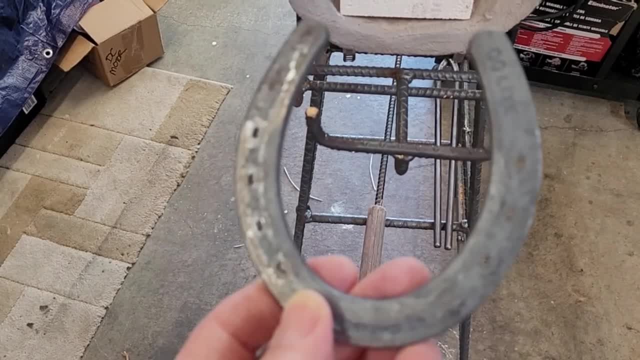 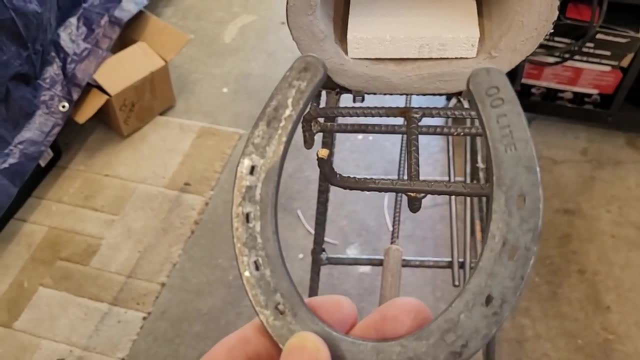 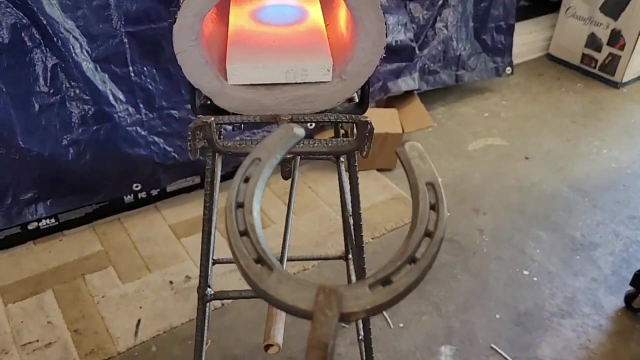 the heat inside the forge and then, once we shut it down, it should take less time to cool down. so anyway, we'll fire it up and give it a try. okay, I'm going to go ahead and put the horseshoe into the forge. I am noticing. 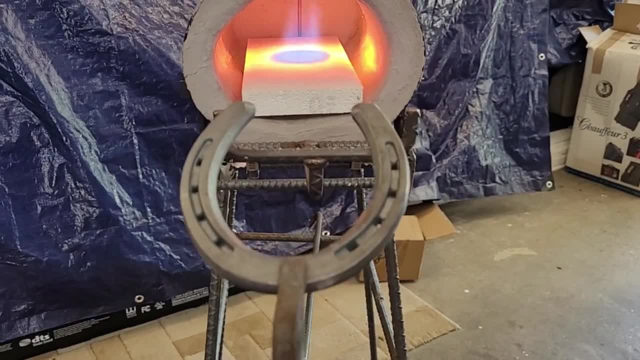 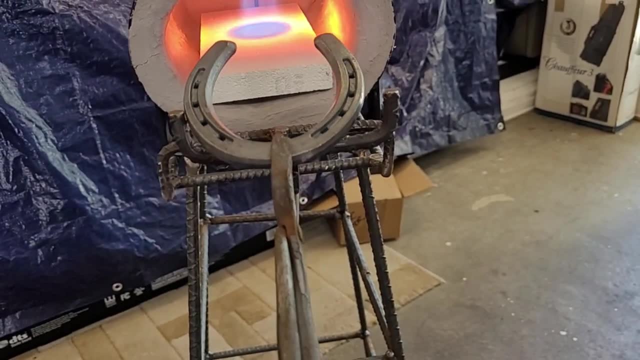 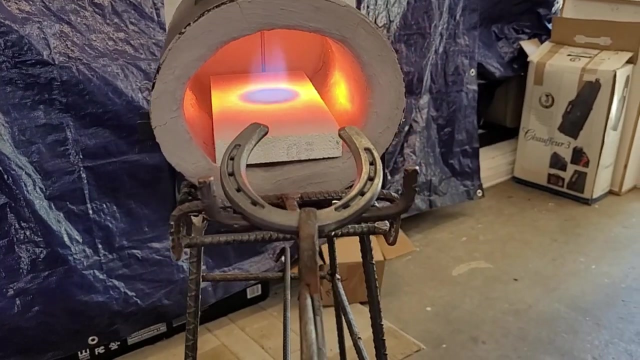 that the insulating brick, the thermal ceramics brick, is actually glowing, which I wasn't expecting it to glow quite as much. but again, we'll see if it makes a difference. we'll put this in and we'll see. we'll see if it makes a difference. we'll put this in and we'll see if it makes a difference. 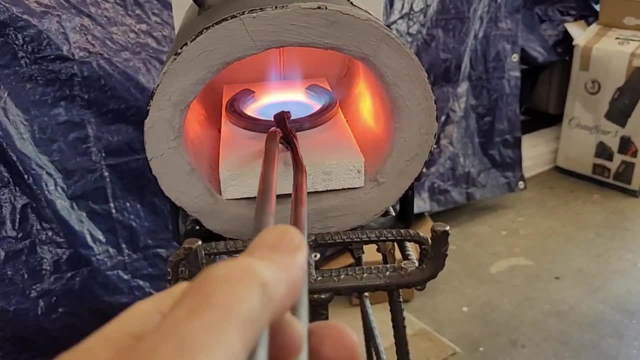 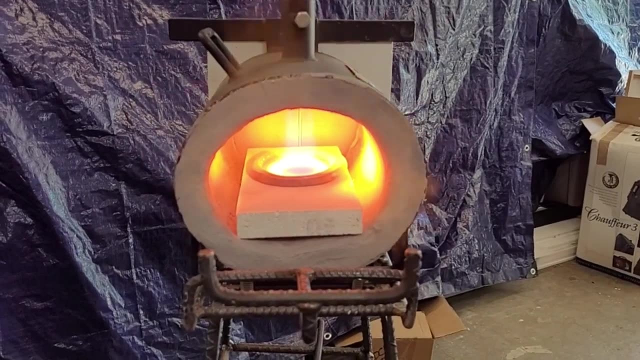 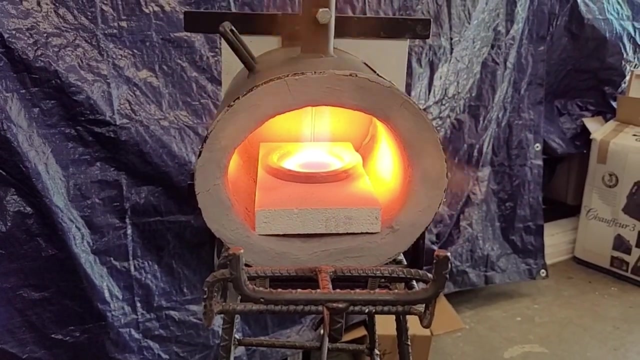 we'll put this in and we'll see if it makes a difference, and I will give you updates over the next few minutes. So we're at the two-minute mark and the horseshoe is coming up to temperature fairly rapidly, so I think within another minute or so. 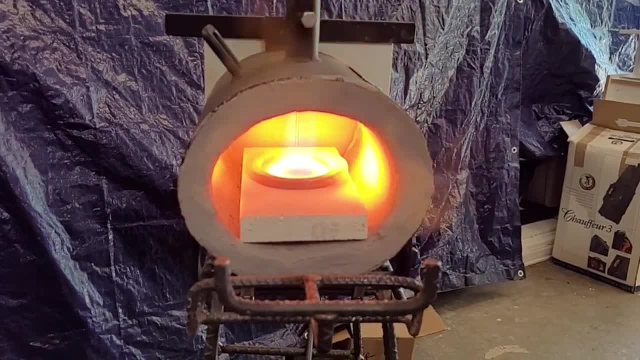 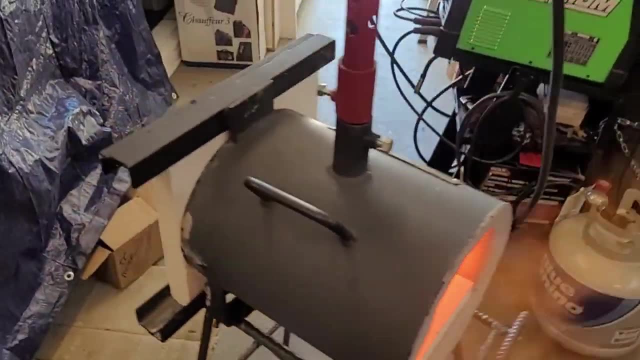 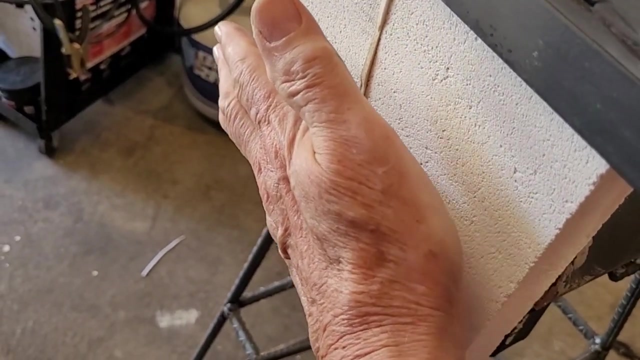 I'd be to a point where I could put it into my bending jig and start working with it. Now, one thing I can say is if you come around to the back and put your hand next to the bricks, you can really feel no heat. 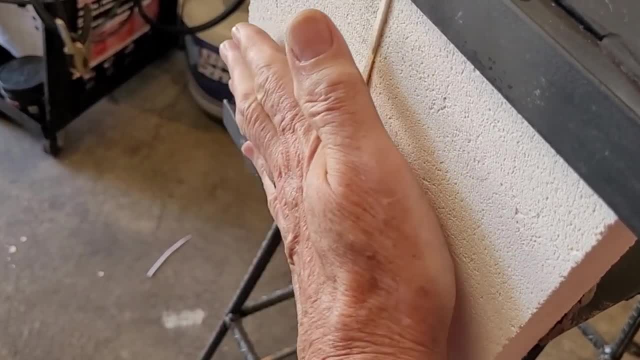 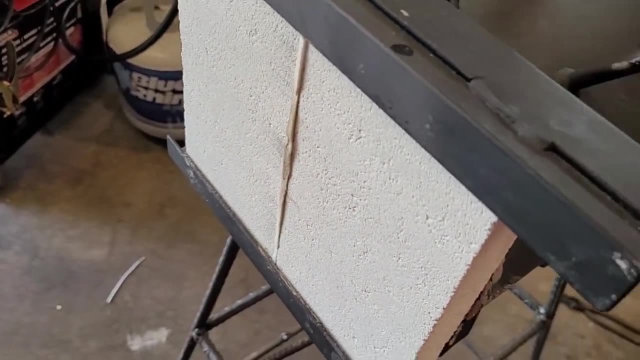 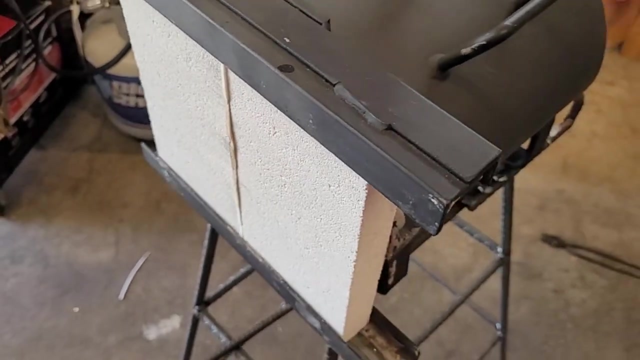 In fact. I mean, I can touch that. It's a little bit warm, but not to the point where if I touch it I'm going to burn myself. So definitely. these bricks have some pretty good insulating properties. So we're at the three-minute mark now. 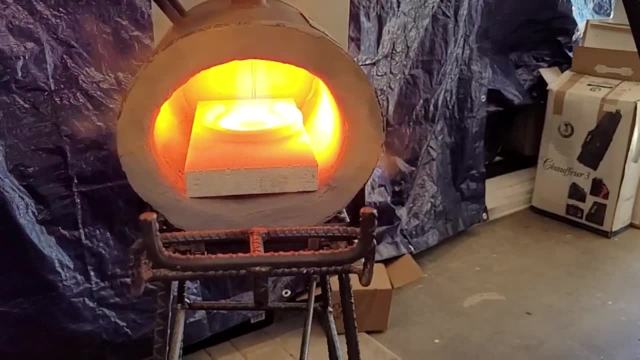 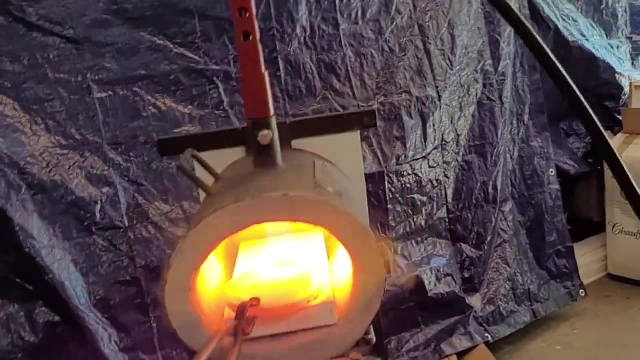 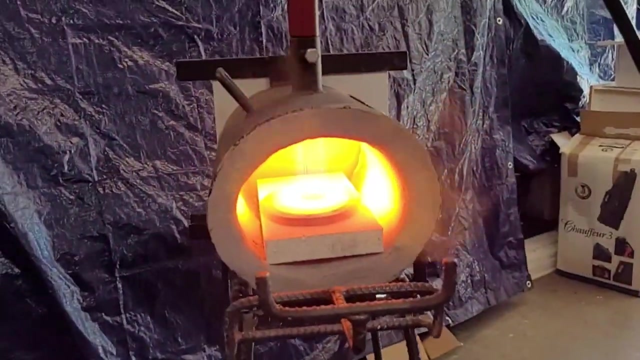 and that horseshoe is definitely up to temperature. This is the color that I normally use. when I'm ready to start bending a good yellow-orange color Again to the back of the forge, I'm going to put my hand next to the bricks. 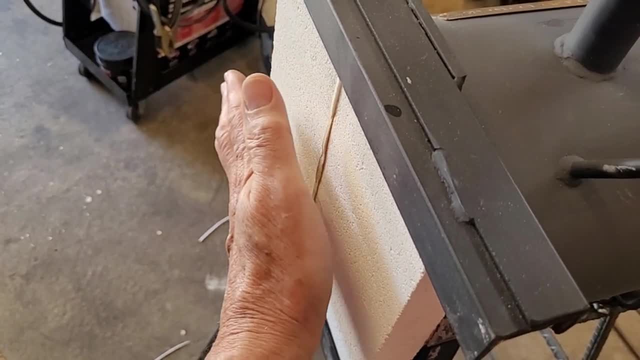 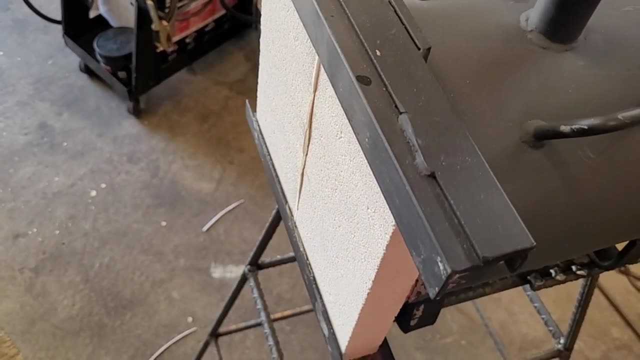 and I'm going to put my hand next to the bricks. In terms of temperature of the insulating bricks, they're a little bit warmer, obviously, but not to the point where I'm burning myself by putting my hand on them. So they do have very good insulating characteristics. 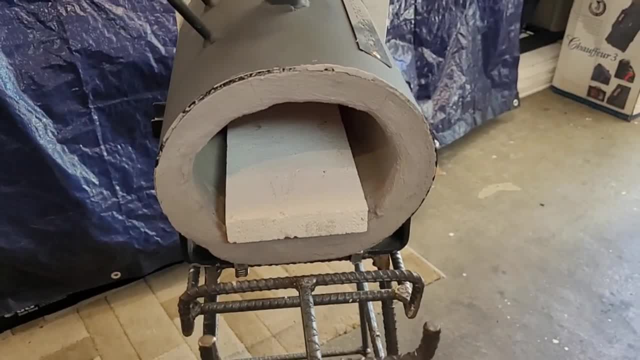 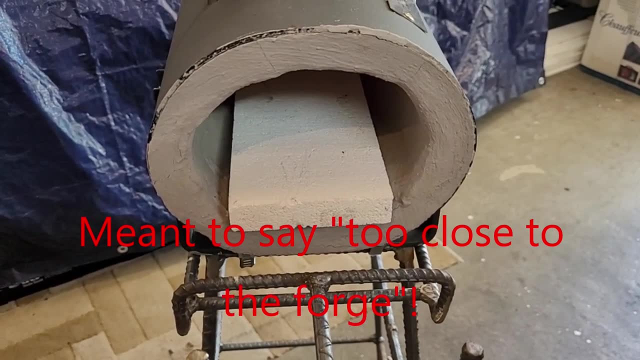 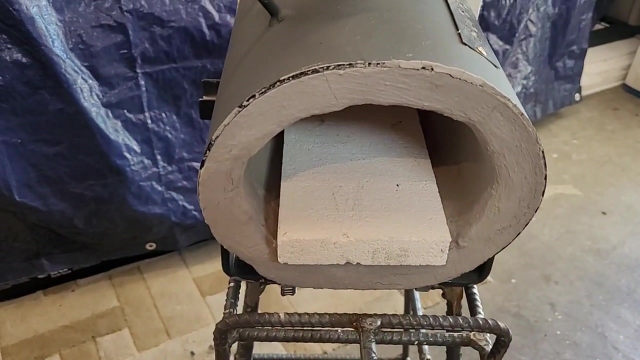 Okay, sorry about that technical glitch. My phone overheated from being too close to the phone, so I had to put it. I had to put it in the freezer for a little bit and let it cool down. But what I was saying was is that the people at IUNO's best recommended. 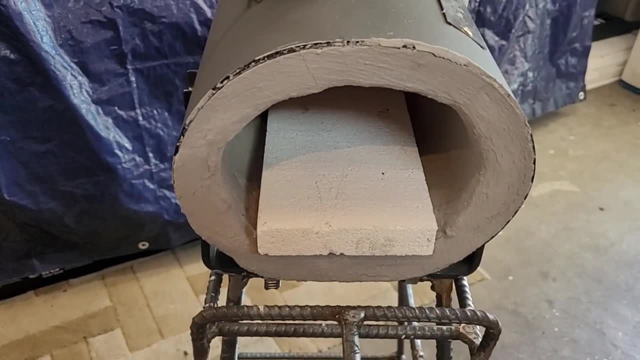 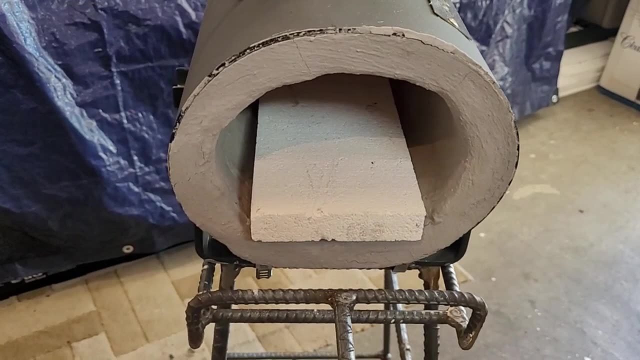 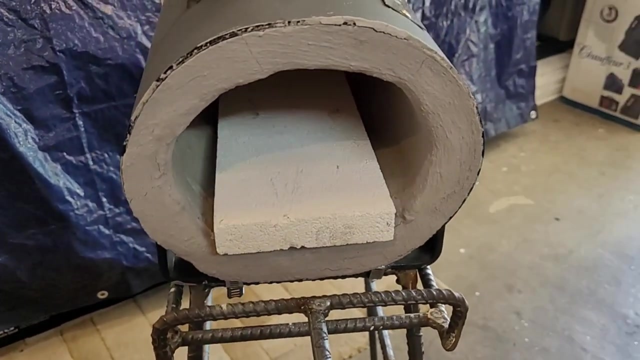 coating the brick, or at least maybe the edges, in a thin coating of the Ka-Bond wet mortar and letting it dry, and it just helped prevent chipping on the edges. Again, these are insulating bricks so they're not going to be as durable as the hard fire bricks. 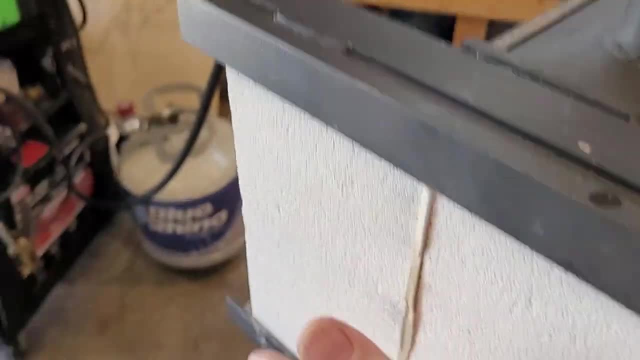 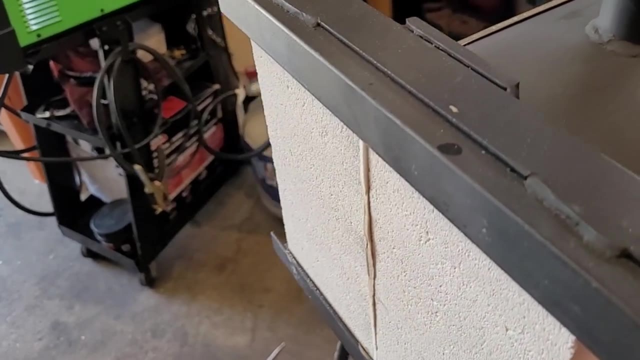 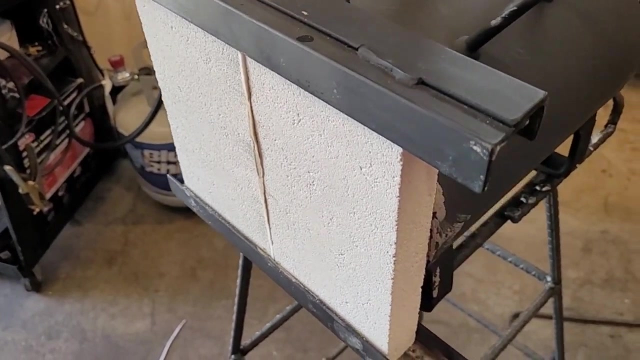 and again back to the back. you know they're warm now. We've been running this forge for quite a while, but still there would be no way I could have touched the regular fireplace fire bricks at this point. I mean, they would simply almost still be glowing red. 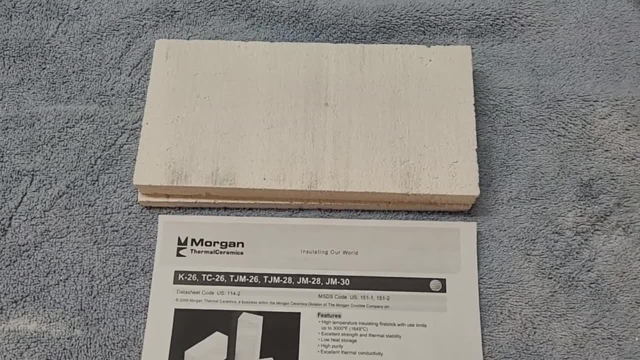 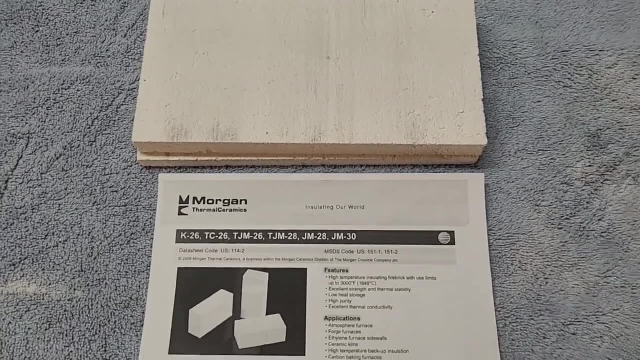 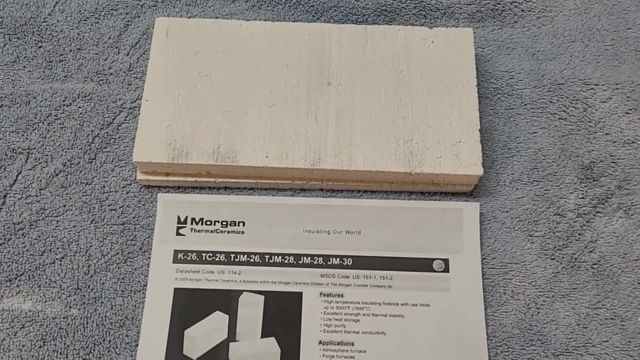 So, all in all, I think I'm going to be very happy with these mortars. These are Morgan Thermal Ceramic Insulating Fire Bricks Pros. they definitely do insulate. I think you can see from this video the insulating properties. 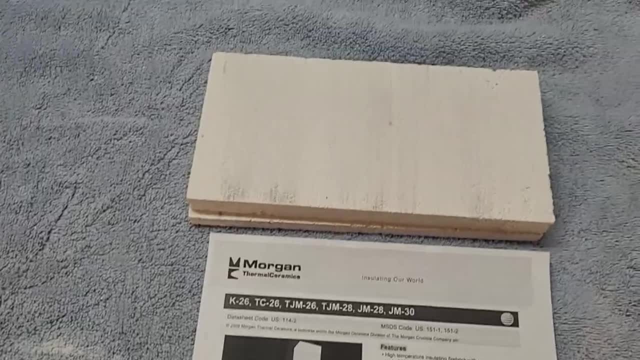 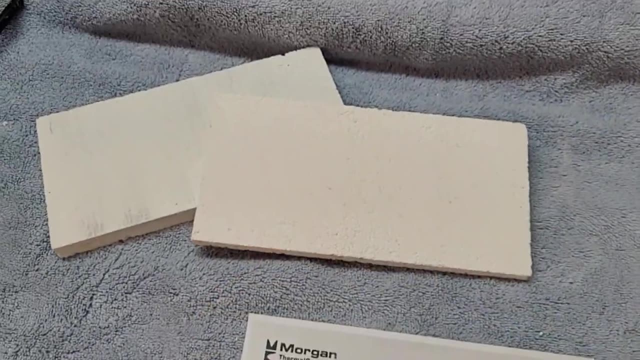 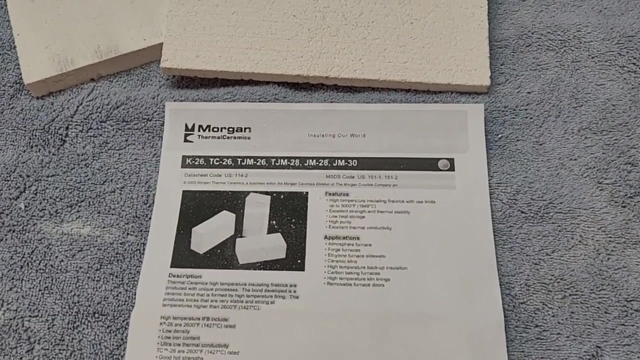 of these fire bricks. They are very light. I mean this half-inch one is like a feather, It is very light. But again, the whole thought is that it's an insulating brick as opposed to a dense fire brick and being able to use these thinner insulating bricks. 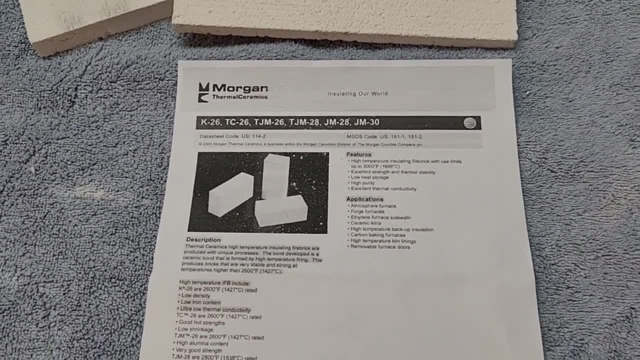 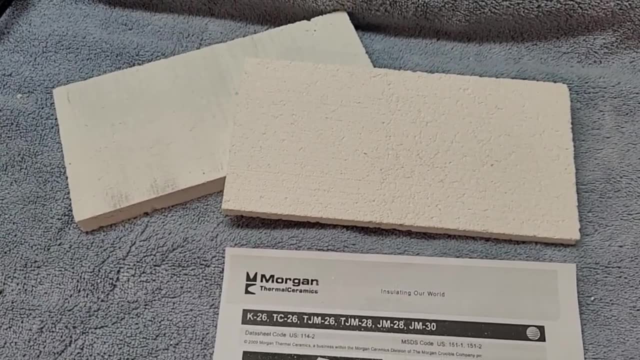 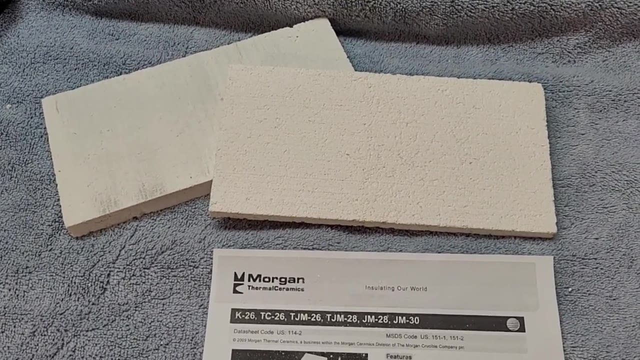 inside my forge gives me a little bit more space to operate. They did seem to perform really well in the heat test for the 00 horseshoe. Typically I said it would take four to five minutes to heat up to temperature in my forge. 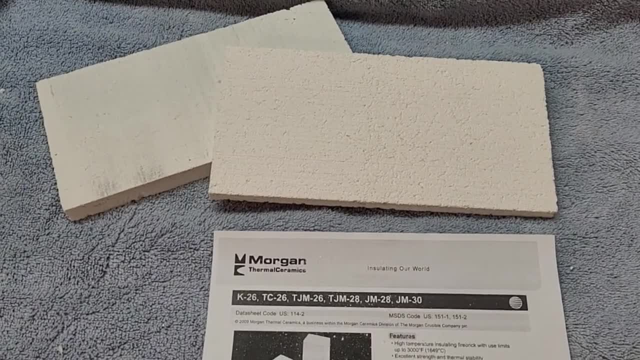 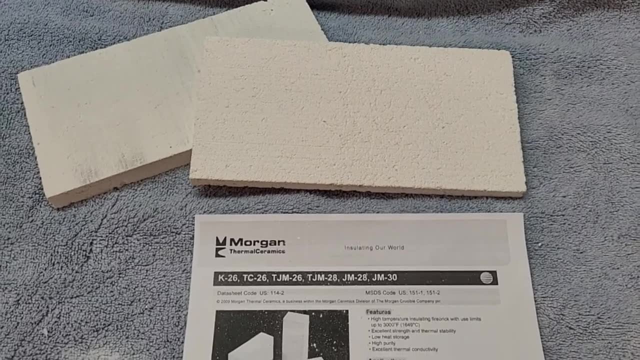 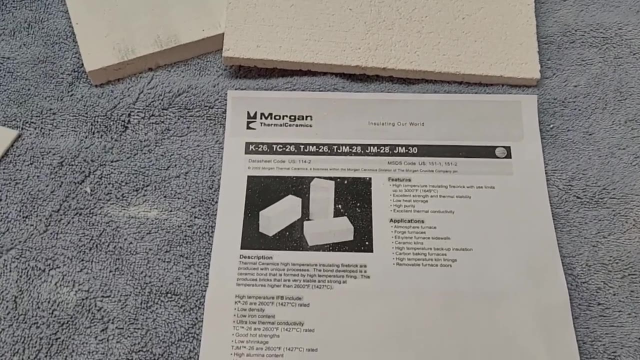 I think you can see at three minutes they were up to temperature. The horseshoe was up to temperature where I could easily bend it in my bending jig, So I think they're going to perform really well. Durability again: they are more fragile. 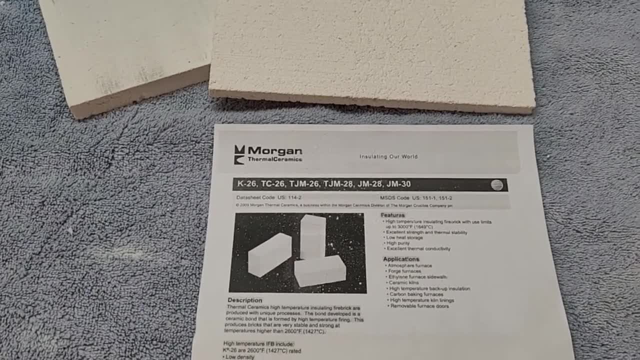 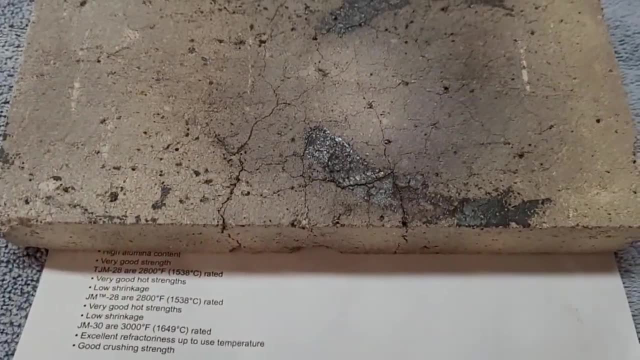 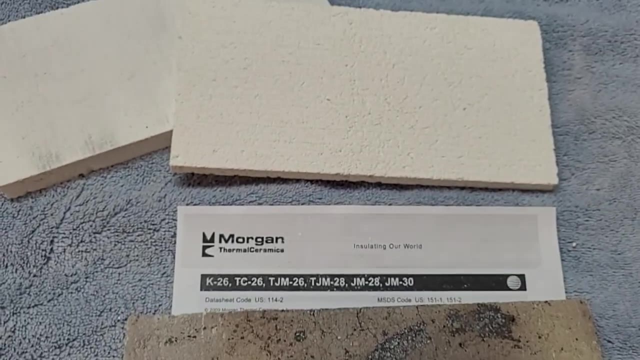 than the regular fire bricks. but one of the things with fire bricks- and I can show you this as an example- they develop lots of cracks And I've had several of them crack completely in two. so I'm anxious to see, given that these are insulating bricks- 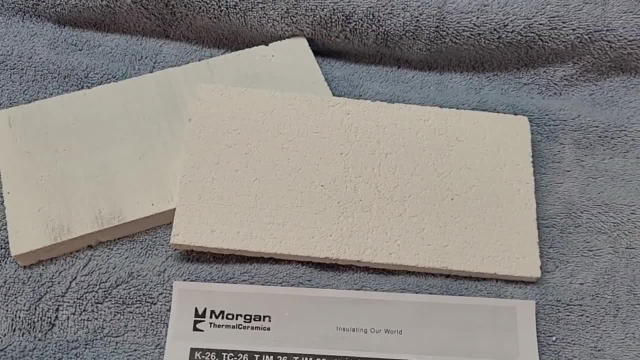 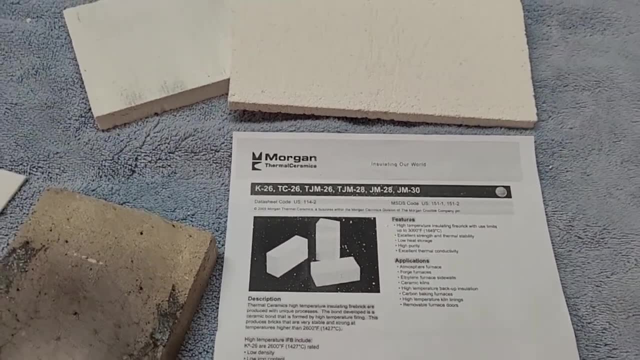 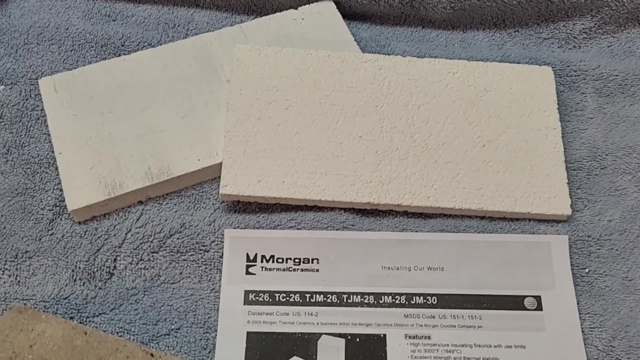 will they suffer from that same problem? I don't think so, but if they do, I will report back Cons. they are more expensive than just the regular old fireplace fire bricks, but I guess you get what you pay for in terms of performance. 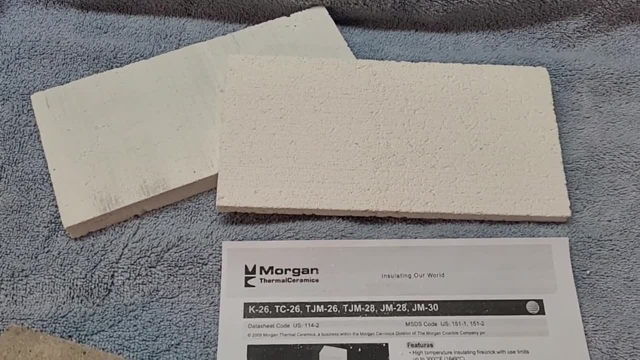 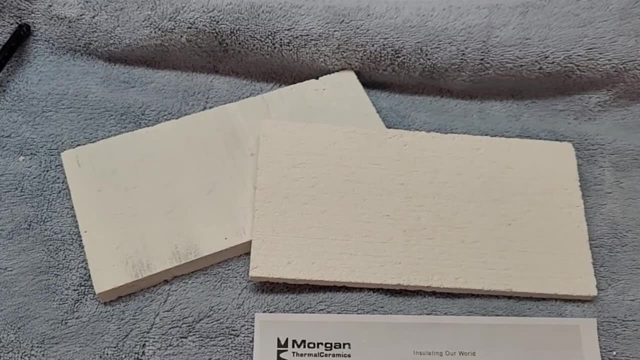 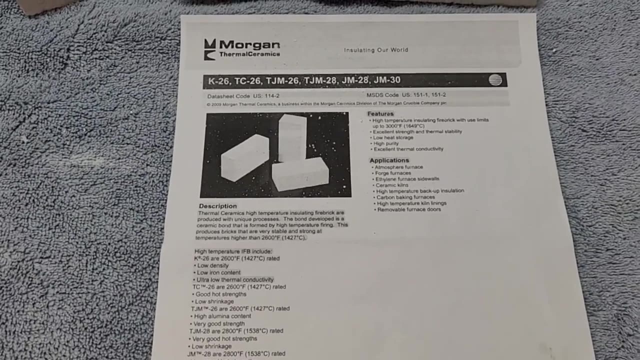 and hopefully longevity of the product. So again, I will post the links to the IUNO's best site and the spec sheet here that I've got, and they've got a whole bunch more specifications on their site. So overall I think I'm going to be very pleased. 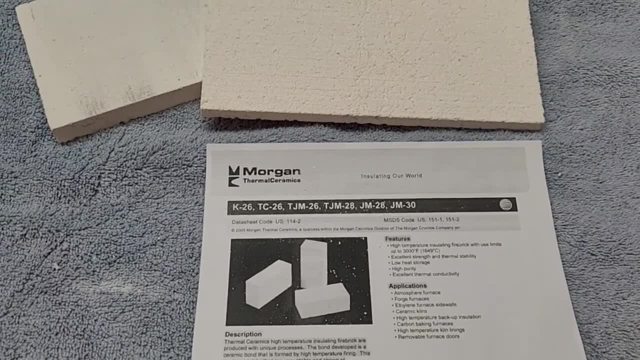 I would highly recommend giving these insulating fire bricks a try.